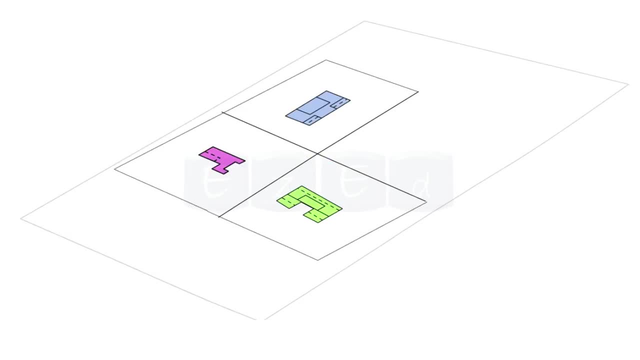 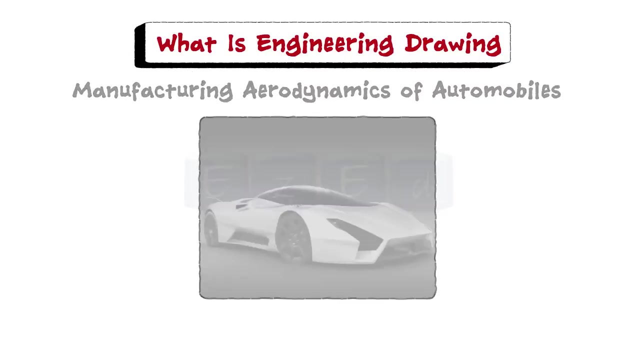 More than drawing pictures. it is also a language, a graphical language that communicates ideas and information from one mind to another. Most important, it communicates all needed information, from the engineer who designed a part to the worker who will make it. Application of engineering drawing is used in ships, manufacturing aerodynamics of automobiles, constructions, etc. 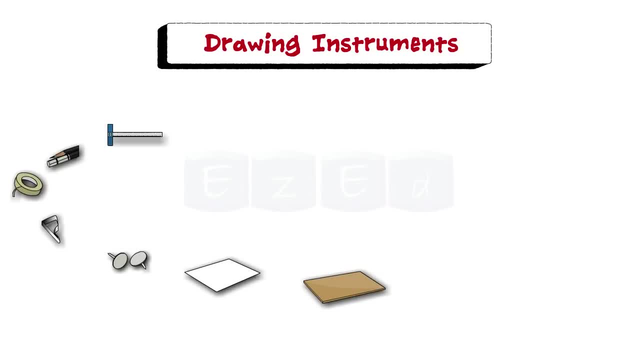 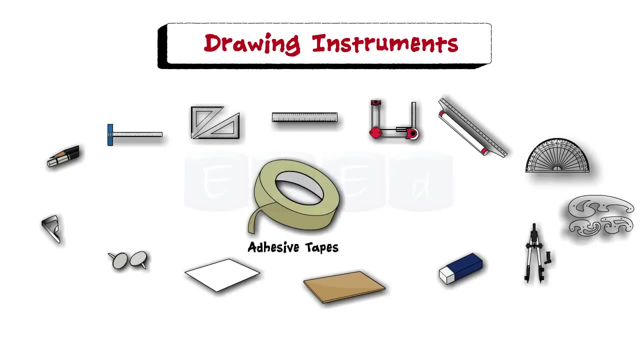 Let us see different drawing instruments used in engineering drawing. In this we have a drawing board, drawing paper, pins, clips or adhesive tapes, pencils, T-square set, square scale drafter, roller scale protractor, french curves, compass and eraser. 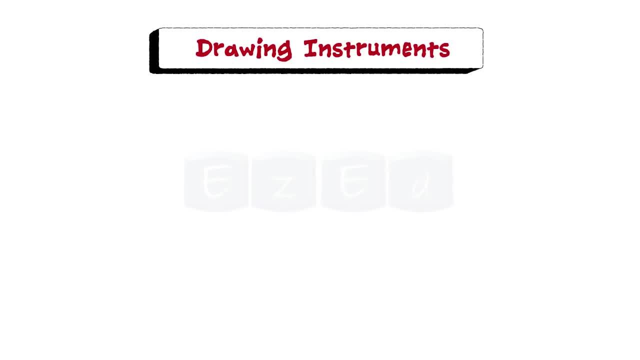 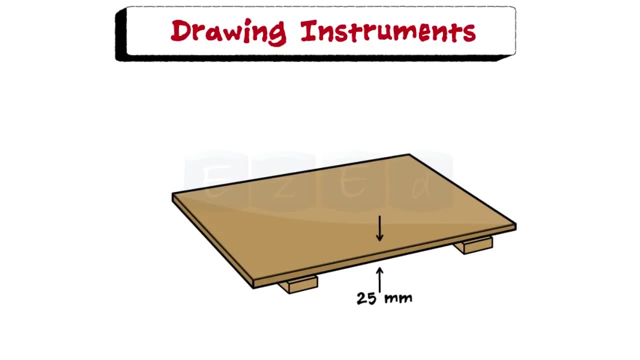 Hey, it's time to concentrate now. Now let us describe each and every instrument. Drawing board is rectangular in shape and is made of wood about 20 mm thick. It is cleated at the back by two battens to prevent warping. 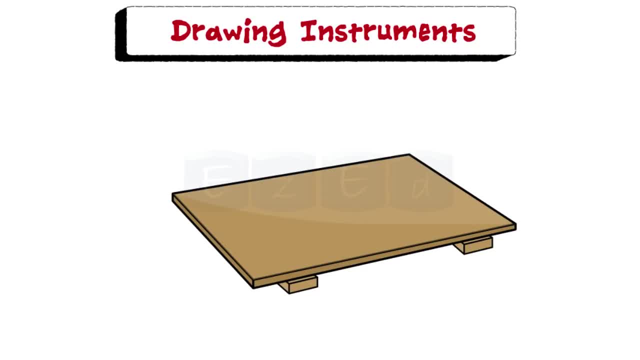 The surface of the board should be smooth and it is used to keep the drawing paper. There is a working edge at the side of the drawing board. While selecting a drawing paper, we have to be sure that the size of the paper is smaller than the drawing board. 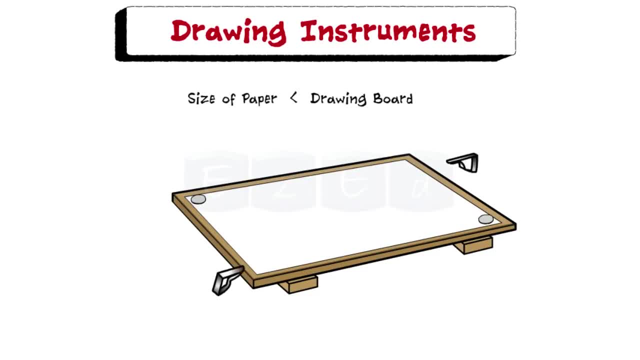 To hold this drawing paper we use pins or clips or adhesive tapes. Pencils are basically used to draw. The accuracy and appearance of a drawing depends on the quality of the pencils used. The grade of pencils- H, 2H and HB are mostly used. 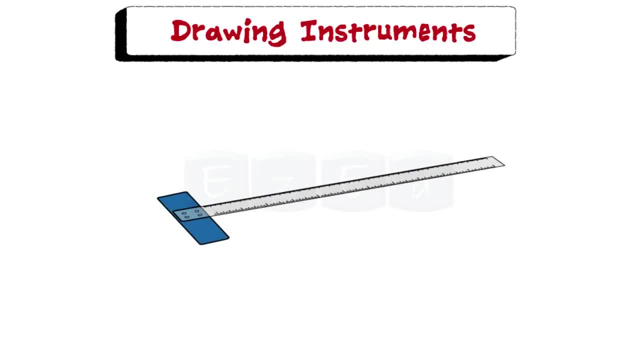 Next is the T-square. It is made of two parts, the stock and the blade, which are joined together at right angles by means of screws and pins. T-square is fitted at the side of the drawing board and it slides along the edge of the board and is used to draw horizontal straight lines. 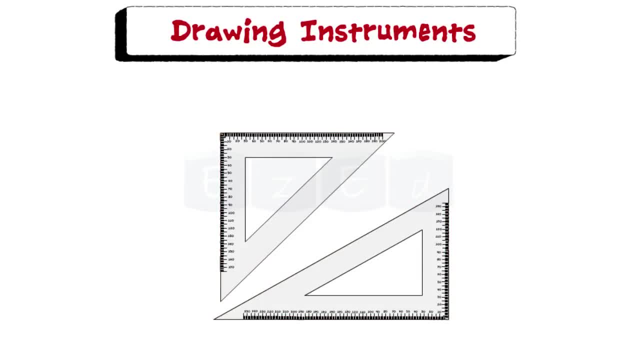 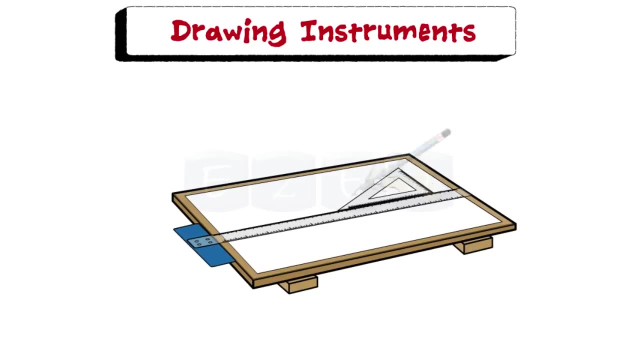 Set-square is triangular in shape, with one of the angles as right angle. Two forms of the set-square are generally used, One having angles 45,, 45 and 90 degree, and the other is 30,, 60, 90.. Set-square is a combination with T-square is used to draw lines at an angle. 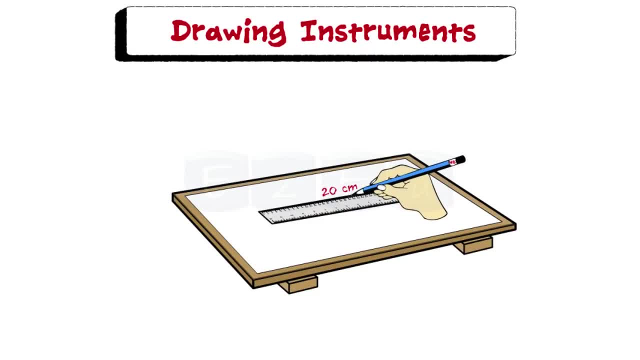 A scale is used to draw lines of specific length. Protractor is flat and semi-circular in shape. Its circumferential edge is graduated to one degree. It has one degree divisions and is numbered at every 10 degree interval and is readable from both the ends. 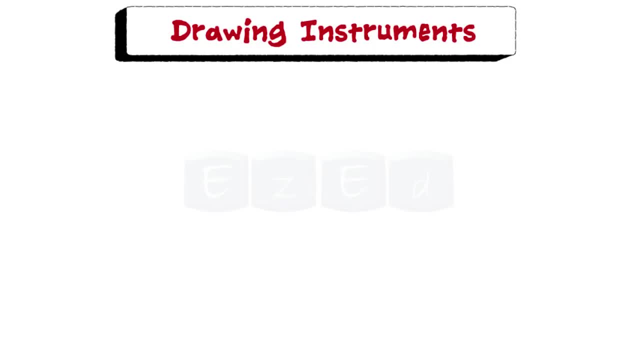 The protractor is used to draw or measure angles. The combination of a T-square, a set-square, scales and a protractor is a drafter. Its one end is clamped by means of a screw at the edge of the drawing board. 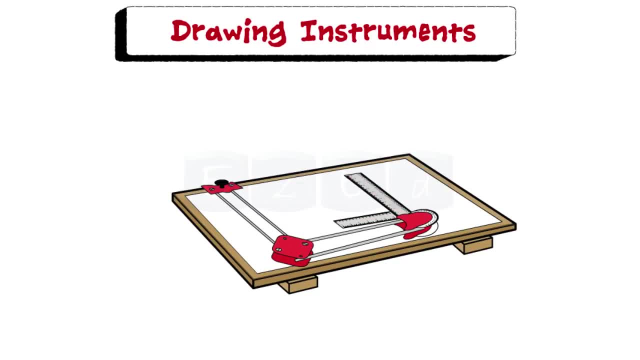 The other end is adjustable. It has a scale which is at 90 degree and also has a protractor which can be rotated at certain angles. This scale can be moved anywhere you want Within its limits. Next is a roller scale. It has a roller in it. 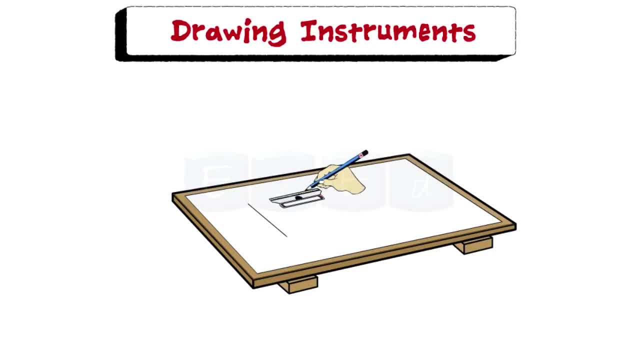 It is used for drawing vertical lines, horizontal lines, parallel lines, angles and circles. Next instrument is a French curve. They are made in various shapes, one of which is shown here. French curve is used for drawing curves which cannot be drawn with a compass. 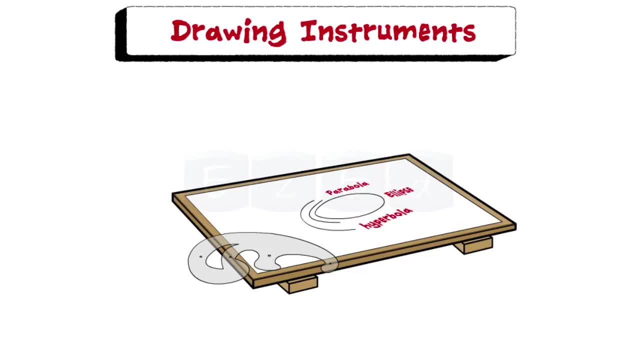 It is used to draw curves like ellipse, parabola, hyperbola, etc. A compass is used to draw a circle of a specific radius and an arc at a specific distance. Soft Indian rubber is widely used to erase pencil drawings. The eraser should be such that it does not spoil the surface of the paper. 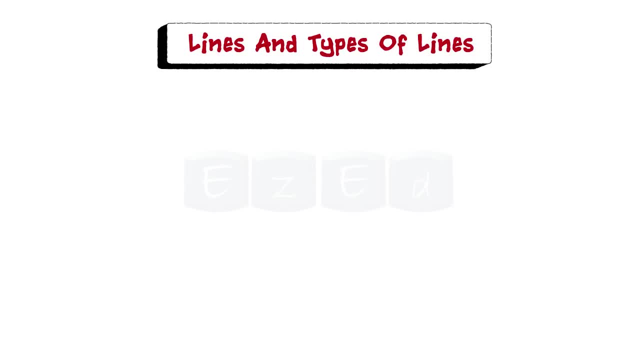 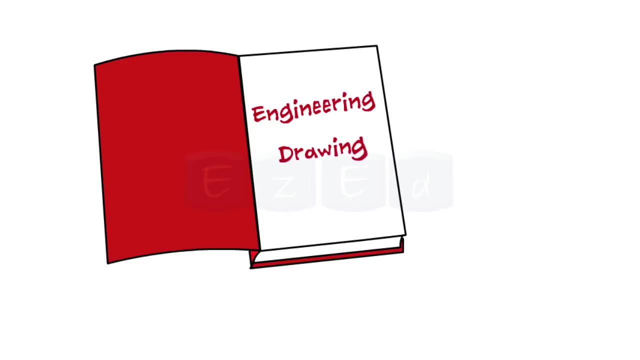 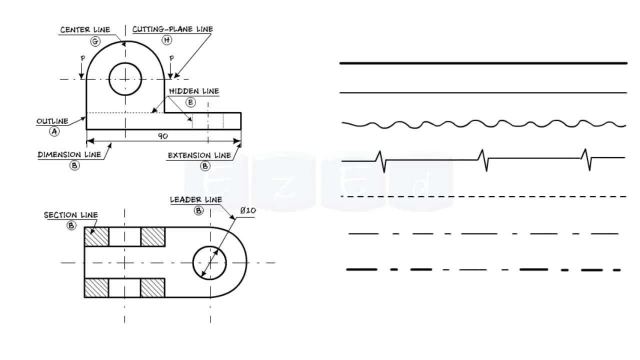 Next we will see lines and types of lines. Just as in any textbook, we are thought to use the correct words for making correct sentences. Similarly, in engineering drawing, the details of various objects are drawn by different types of lines. Various types of lines are used in engineering drawing. 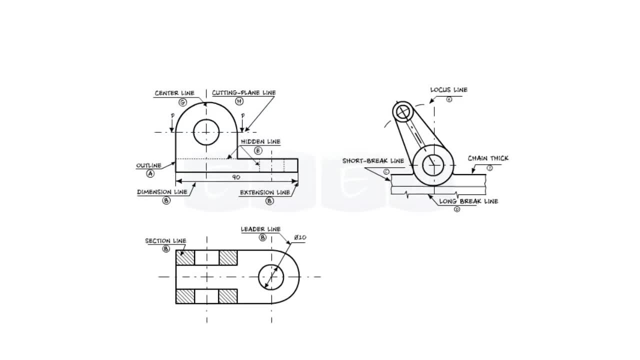 Now let us see the different types of lines. First is a continuous thick line. This line is used to display outline and edges of the main drawing. Next is the continuous thin line. This line is basically used for dimension extension, projection, leaders, hatching, etc. 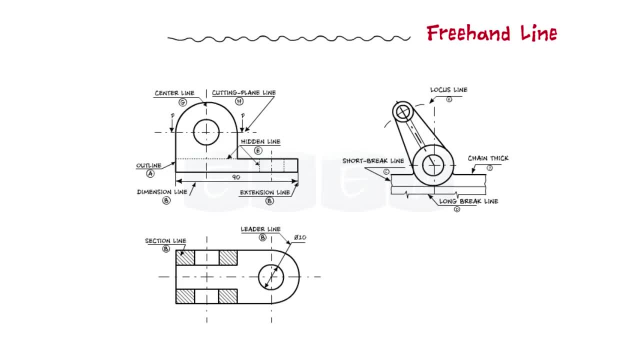 Next is a continuous thin freehand line. This line is used to show short break or irregular boundaries. Next is the continuous thin line with zigzags. This line is used to show long break. Next is the dashed line. This line is used to show hidden edges of the main object.